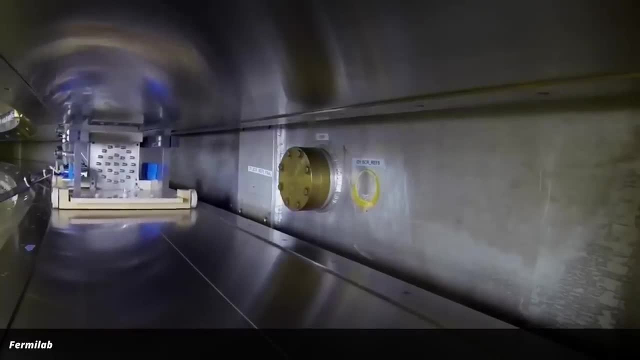 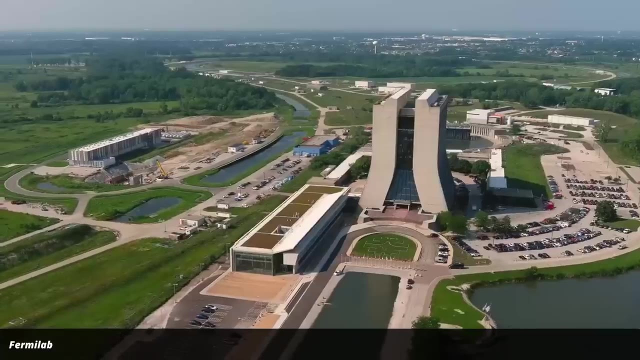 But unlike Twitter threads, which just decay into obscurity, muons decay into other particles of which one can measure the momentum, and from that you can infer the g-2.. Already, in 2001, an experiment at Brookhaven found that the measured value of the muon 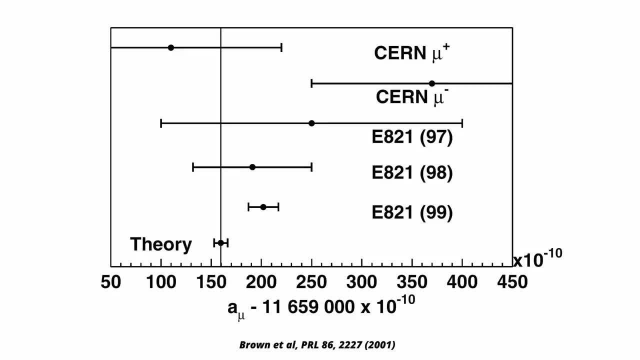 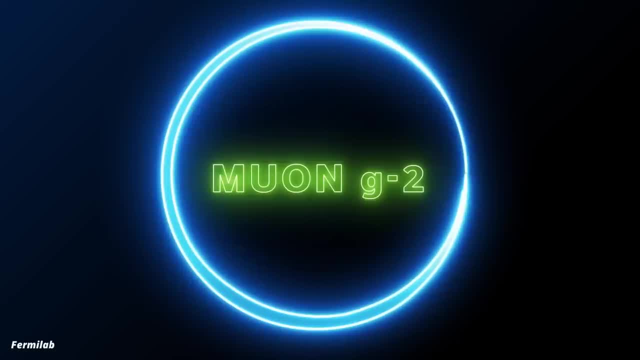 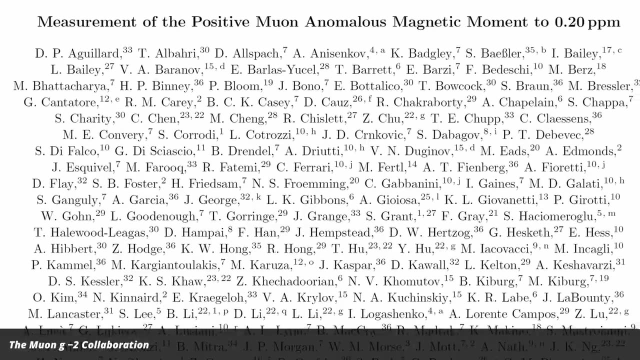 g-2 deviates from that predicted by the standard model, though it wasn't a huge deviation. In 2021,, a follow-up experiment at Fermilab confirmed the earlier result, raising the statistical significance to 4.2 sigma. Last year in August then, the Fermilab group released more data and confirmed the anomaly. 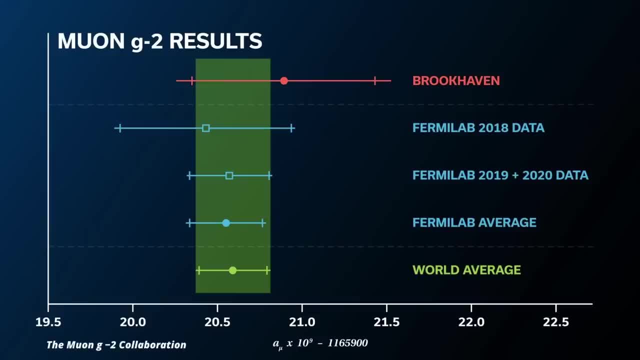 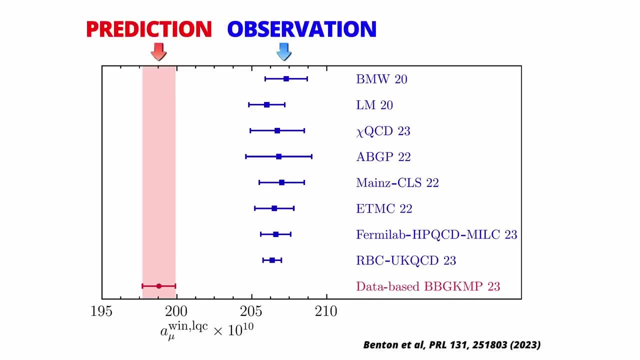 they'd previously measured. The additional data decreased the uncertainty of the measurement and increased the significance to 5 sigma. that's less than a one-in-three-million chance of it being a fluctuation That the statistician was right. statistical significance of the result is now so high means that the discrepancy between 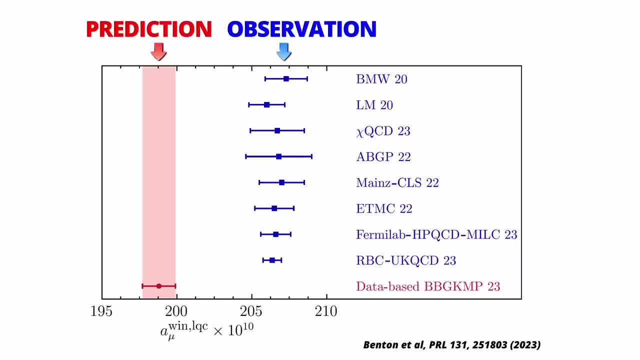 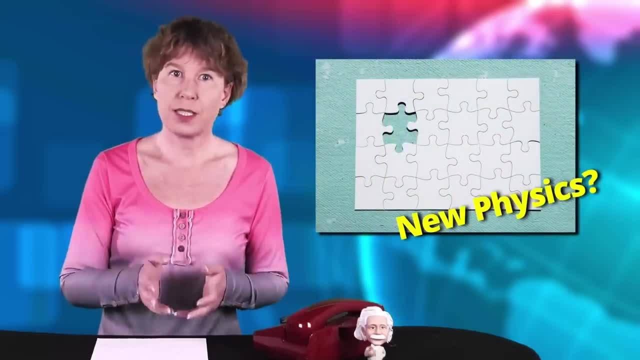 the prediction and the observation is very unlikely to be due to a measurement error. It could mean that something is missing in the standard model, maybe new particles or other new physics. And since the standard model contains three forces, and then there's gravity, which makes 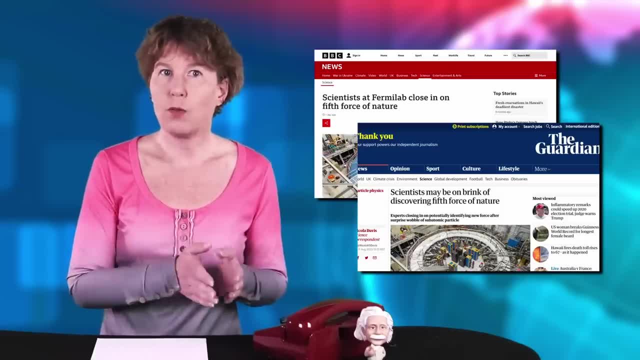 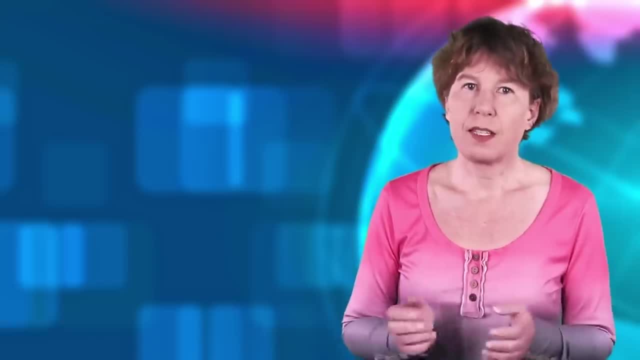 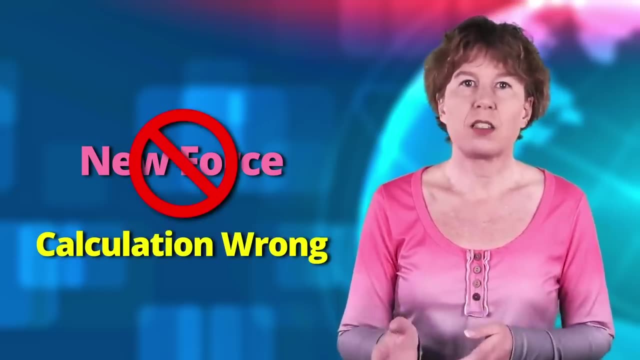 four. in the media they often call the possibility of new physics a fifth force. I explained in an earlier episode what that means. I've always suspected that the discrepancy isn't due to a new force, but a problem with the calculation. This is because these calculations are really hard. 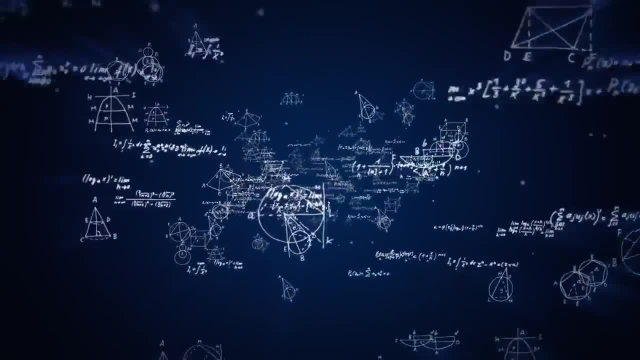 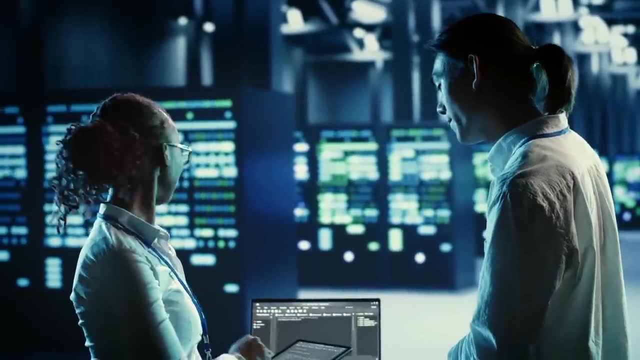 It's not just because it's a lot of mathematics, it's also because in parts we don't have the mathematics, So physicists just do the maths approximately on a computer with what's called a lattice calculation. This opens another can of worms, because how do you know that these are? 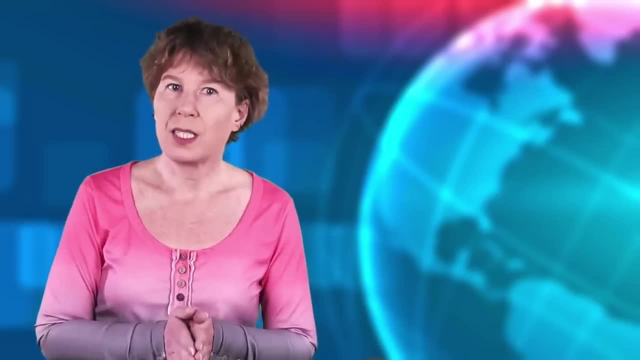 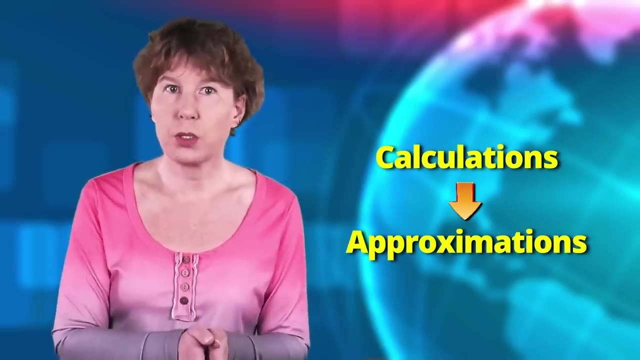 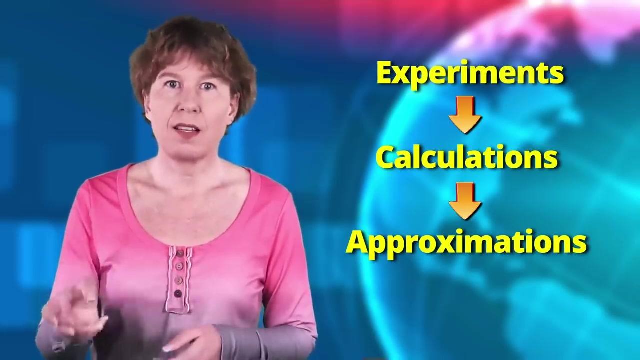 approximations, Are they even good? And in case you thought that's complicated already, there's another complication because all these calculations require further input that needs to come from other experiments. So first you need to extract some numbers from other data and then that goes into your 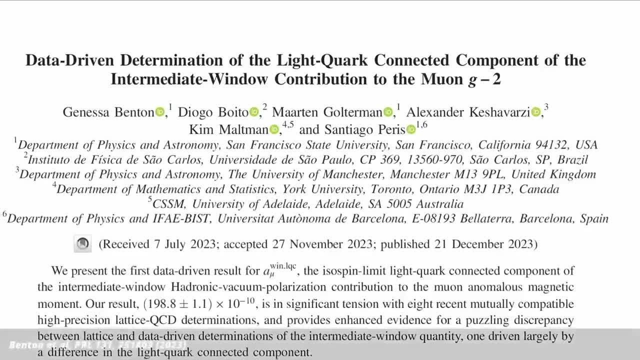 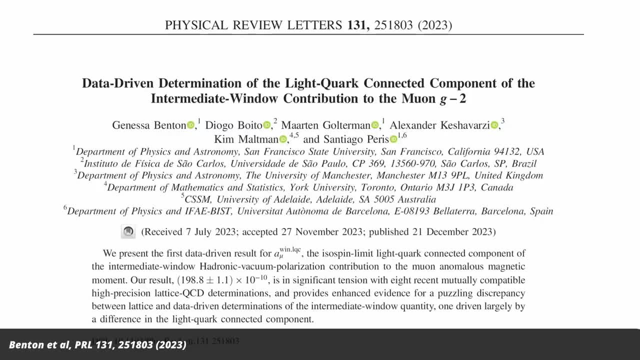 calculation, of which you then do an approximation. And that last bit, the input from other experiments, seems to be the problem. The authors of the new paper have re-calculated this problem. The authors of the new paper have re-calculated this problem.